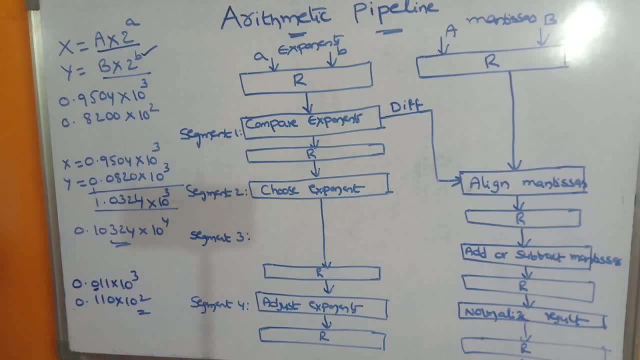 Here we are assuming the base value as 10.. Let the second number is like this: 0.8200 into 10, power 2.. Let us assume that we want to perform floating point addition operation Here. the fastest step is here. after performing the addition, the resultant exponent will become the higher value. 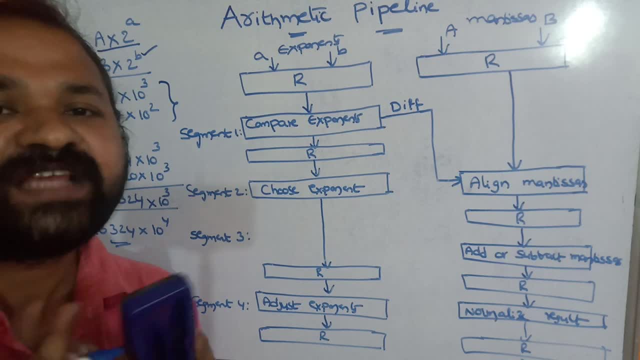 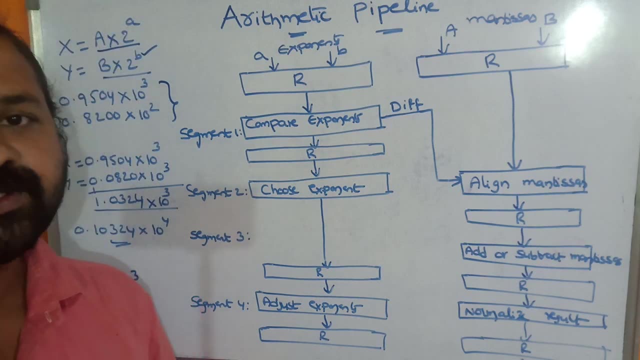 So, between 3 and 2, which is the higher exponent, 3 is the higher exponent, So the resultant exponent will become 3 now So here the step 1 is: we have to compare, we have to find out which is the lesser mantissa value. 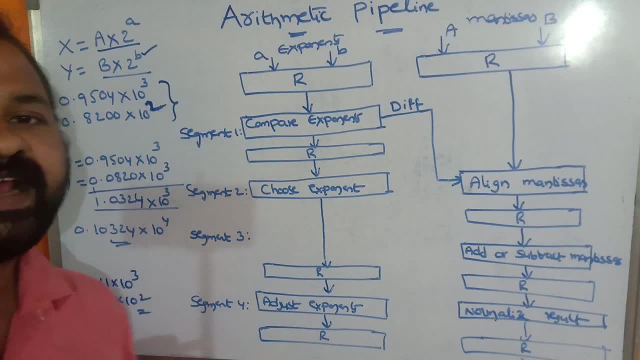 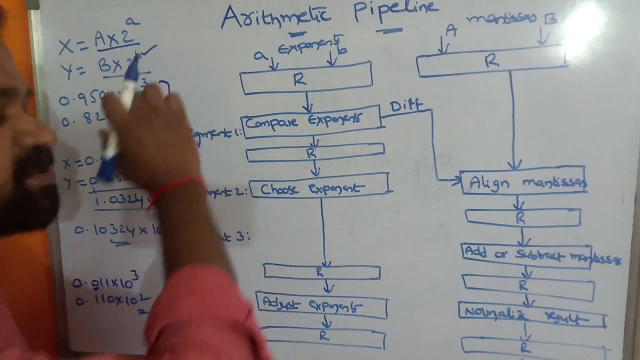 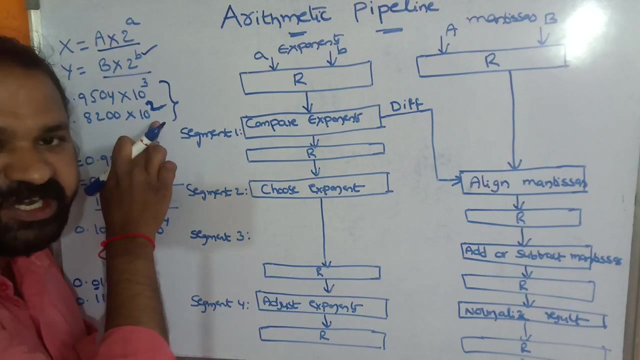 So lesser exponent value. So here 2 is lesser exponent value. We have to align the mantissas in such a way that the exponents must be equal. Here the exponent is 2 here, So we need to perform shift right operation on this number by incrementing the exponent value. 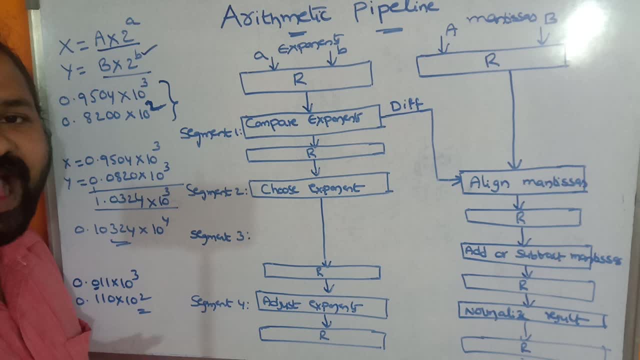 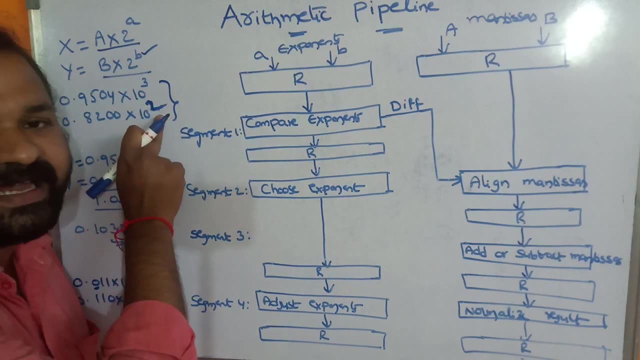 Why? because the difference between 3 and 2 is 1.. So we have to perform shift right operation by shifting one position to the right and by incrementing exponent value. So here the first number is like this: 0.950 into 10 power 3.. 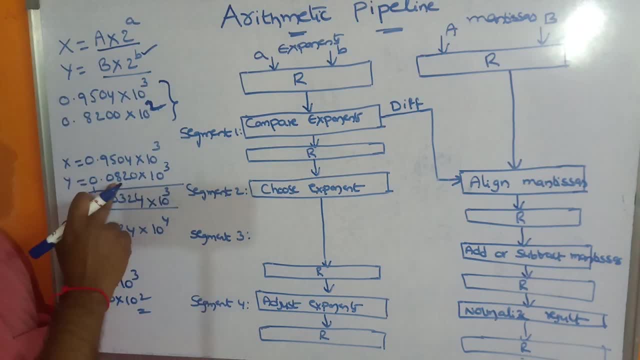 There is no need to make any change on the first number exponent. So now we have to perform shift right operation on the second number by shifting the number one position to the right. So here shifting right means 0 will be appended to the left side and all the bits are shifted one position to the right. 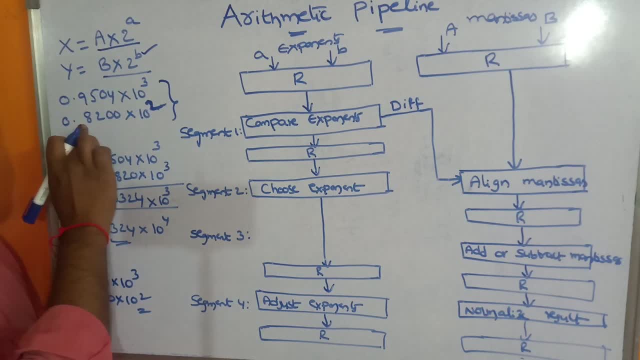 So here we have appended 0 at the right side and all these bits are shifted one position to the right. So 8 is shifted, one position to the right, 2 is shifted, one position to the right, 0 is shifted, one position to the right. 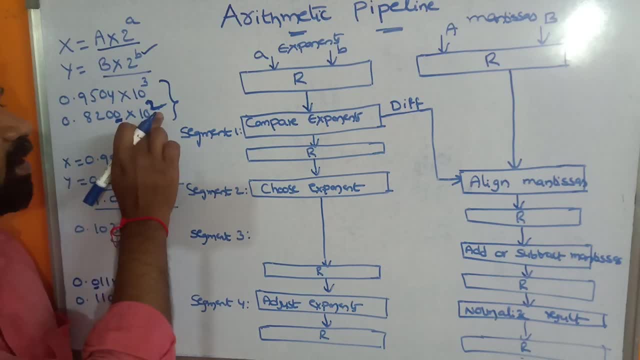 So this rightmost 0 will be discarded into. now we have to perform the incrementation of the exponent, So 10 power 3.. So here exponent is nothing but 3 only, And after that we have to add the mantissas. 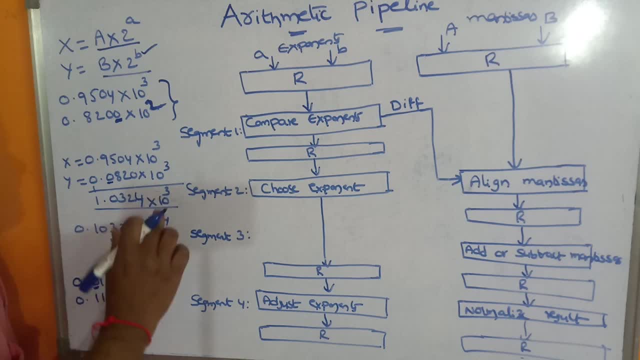 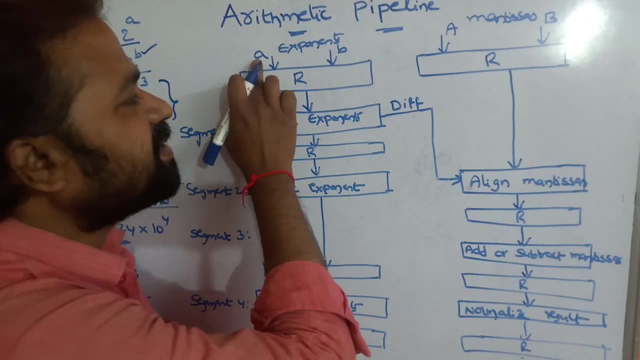 So after adding the mantissas, we got this as the result. So in this way we can perform addition operation on two floating point numbers. Now let us see this flow chart. Here the exponents are a and b, Which are stored in a register called R. 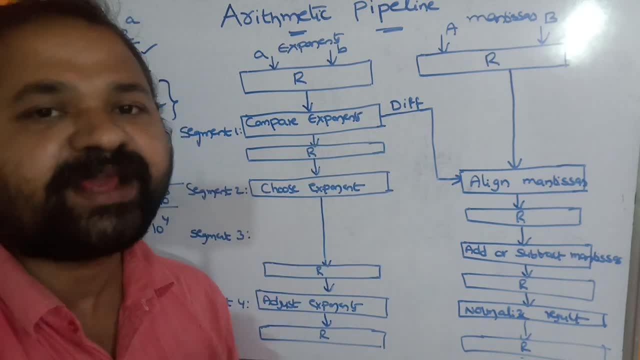 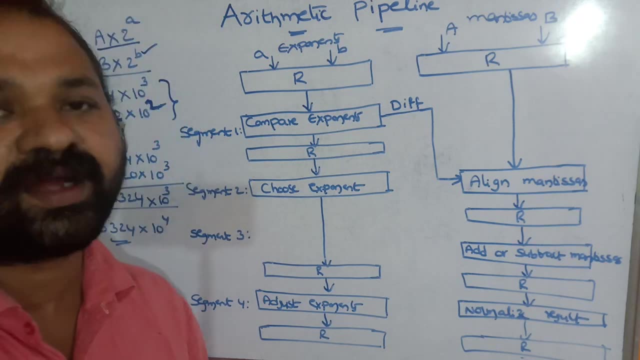 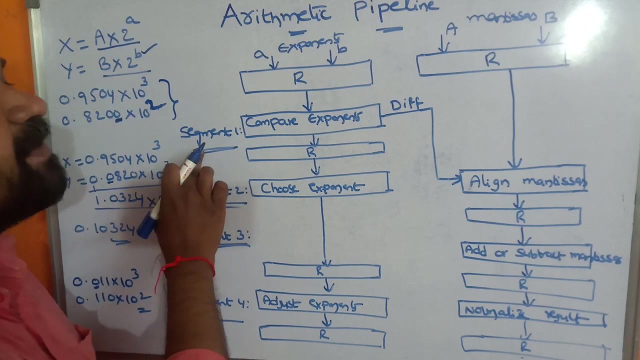 Here R is a register which is useful for the storage of information, And in order to store the mantissas, capital A and capital B, we are using a register called R. Here we are performing the operation based upon four segments. Segment one is compare the exponents. 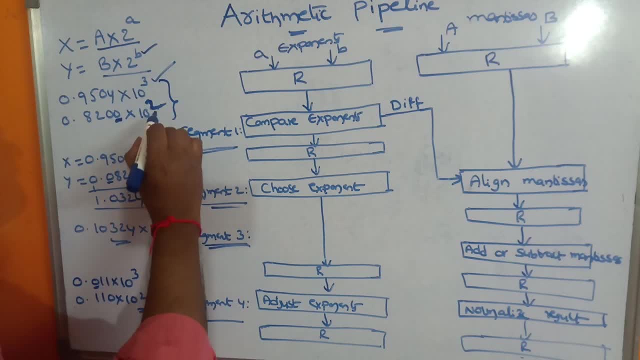 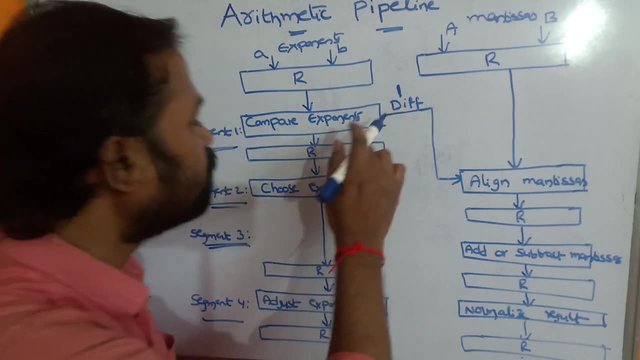 So what are the exponents here? The first number exponent is 3.. The second number exponent is 2.. So the difference between 3 and 2 is 1.. So the difference between 3 and 2 is 1.. So here we have to perform this operation based upon these four segments. 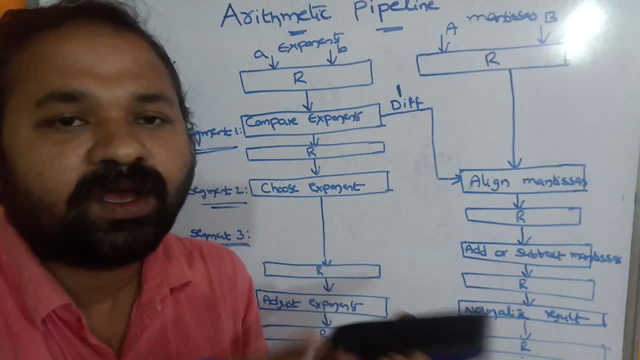 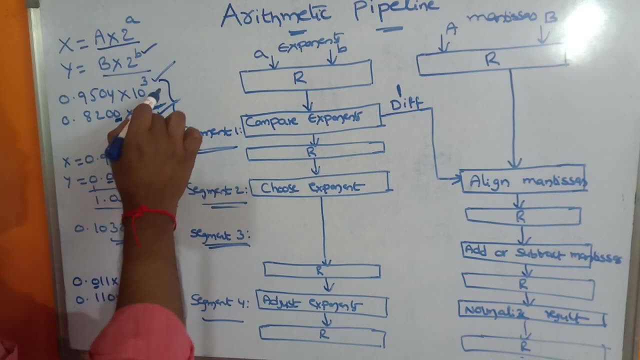 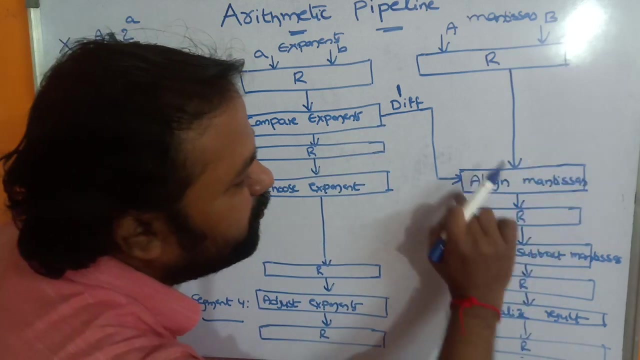 So the entire largest segment is divided into four segments. So what is segment one? Compare the exponents by performing subtraction operation. So the difference between 3 and 2 is 1.. So the difference will be given as input to the second segment. 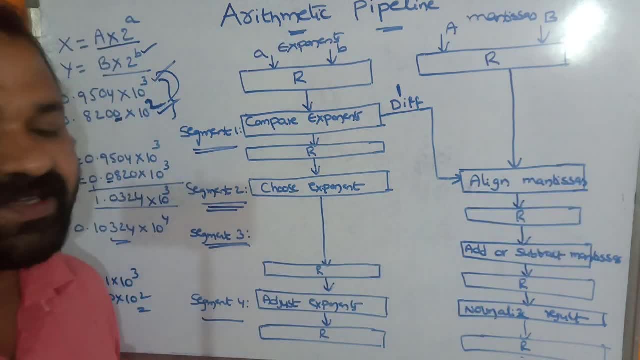 Here the second segment is align the mantissas. So we have to align the mantissas. So how we can align the mantissas here, The difference between them is 1 here, So we have to perform shift rate operation. on the second number. 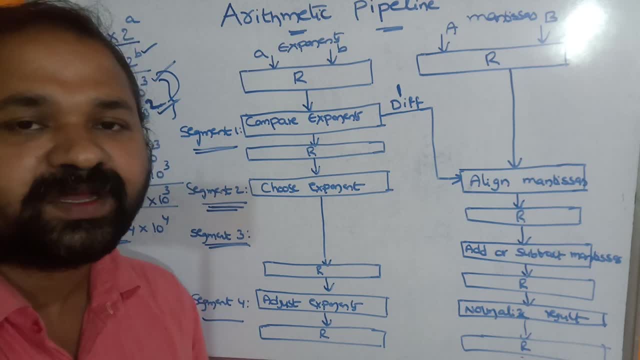 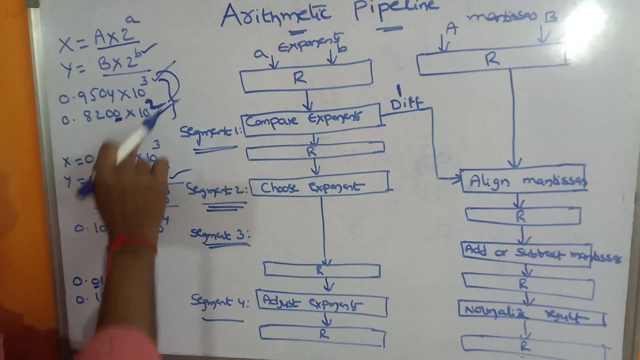 That is the number with lower exponent value- by incrementing the exponent value. So here we perform that operation, Shift rate operation and by incrementing the exponent value. So this is segment 2.. Segment 2 is alignment of mantissas as well as choose the corresponding exponent. 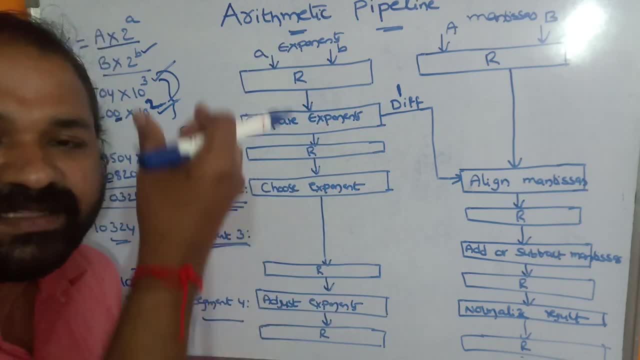 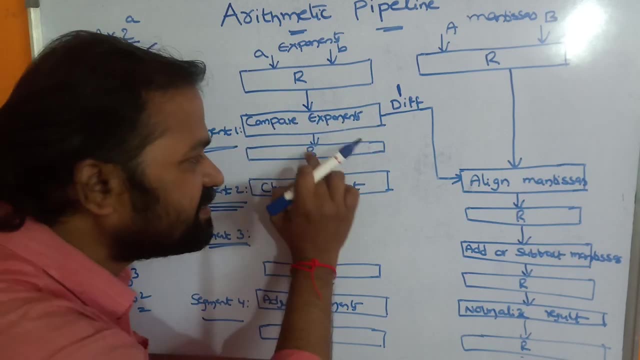 Here: once a segment is over, then we have to store that result in the register. So once segment 1 is over, then we have to store the result in register R. So segment 2 is over. Now what is segment 2?? Align the mantissas. 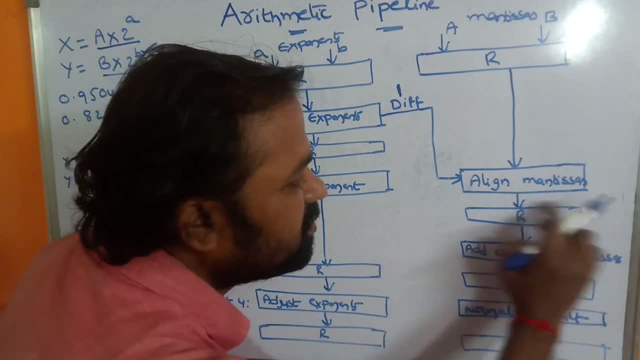 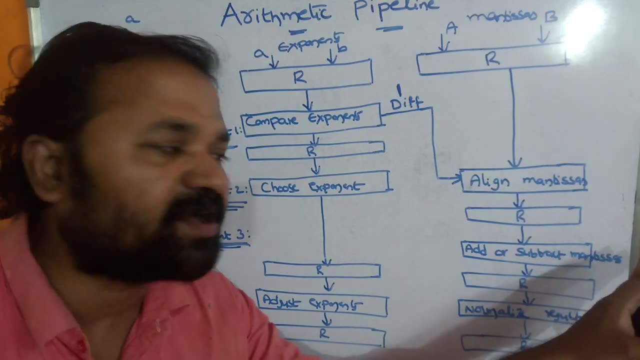 So once alignment of mantissas is over, store the result in register R. Now let us see above. Now let us see about segment 3.. Here the segment 3 is add or subtract mantissas. Let us assume that here we are performing addition operation. 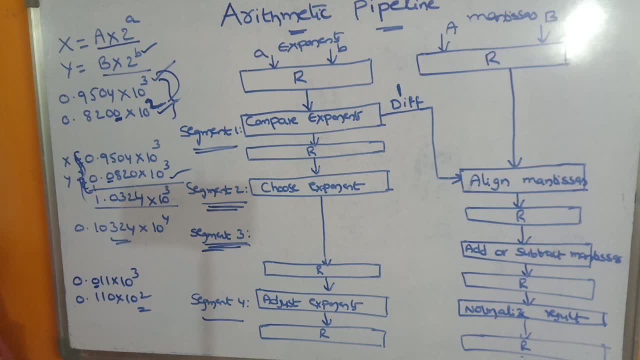 So addition operation means we have to add the exponents So in segment 3 here. so once it is over, then we have to store the result in register R. So here the exponents are stored in this register, as well as mantissas stored in this register. 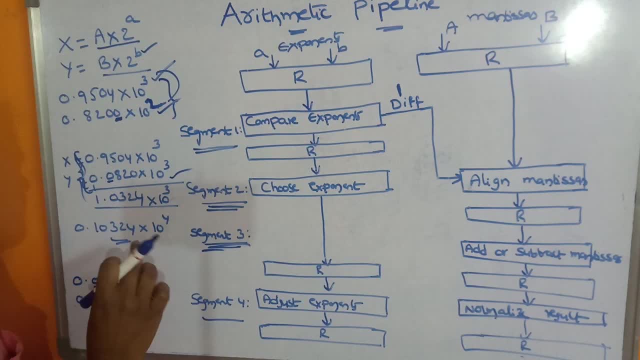 Here. we are not performing anything here on exponents In segment 3. what we are doing Just, we are simply adding the mantissas values. Now let us see about segment 4.. After performing addition operation, there is a possibility that we may get some overflow. 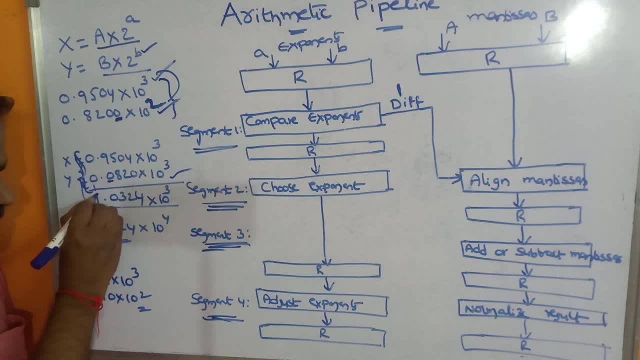 So what is overflow here? Here we have performed the addition operation Here after dot, So before dot. So what is the most significant bit here? 1.. So if the most significant bit here is 1, this before dot, then we can say that there is a overflow. 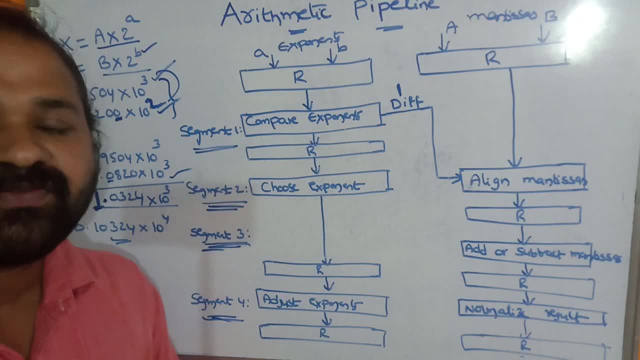 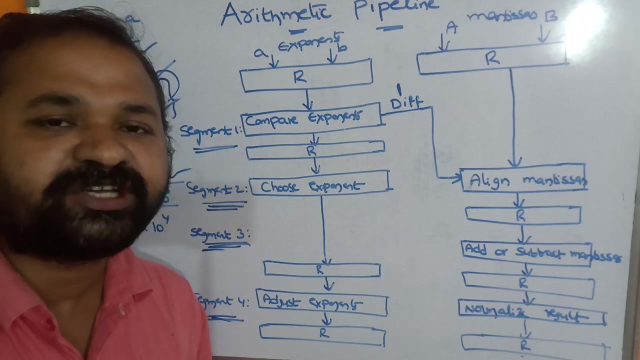 Overflow means the register cannot store that bit. So whenever overflow occurs, then we have to adjust the exponents. That means we have to normalize the result. So how we can normalize the result here: Whenever a overflow occurs, then we have to perform shift right operation by incrementing the exponent value. 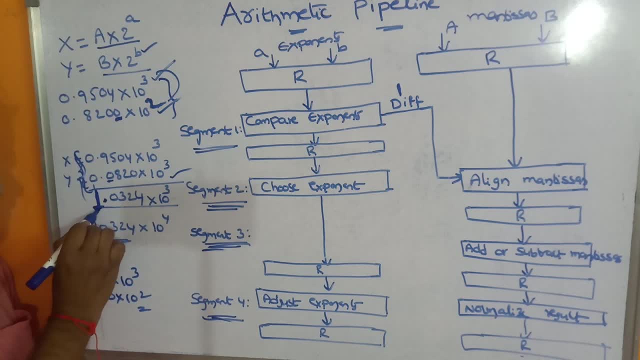 So perform the shift right operation. So this 1 will be shifted one position to the right. So this 0 will be shifted one position to the right. This 3 will be shifted one position to the right. This 2 will be shifted one position to the right. 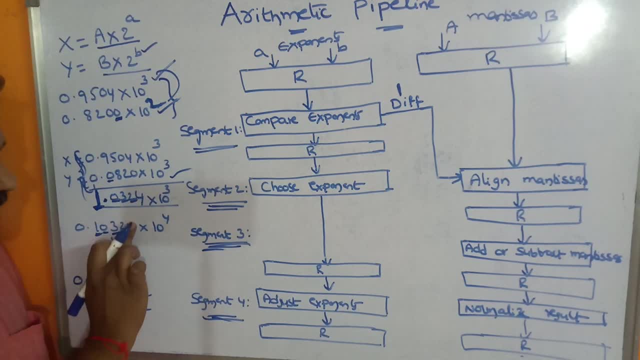 Let us assume that we can eliminate this one. Why? because if you perform shift right operation, then the rightmost bit will be discarded. This exponent will be incremented into 10 power 4.. So this is the result now. So in this way we can normalize the result. 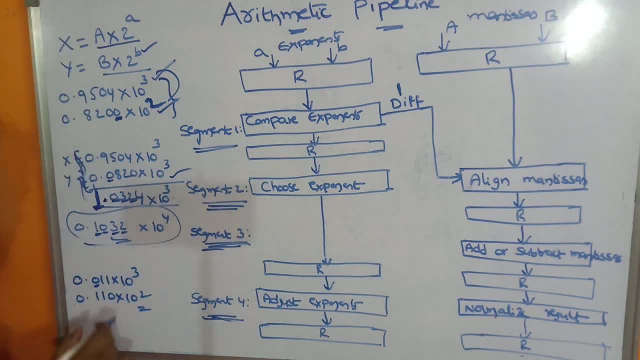 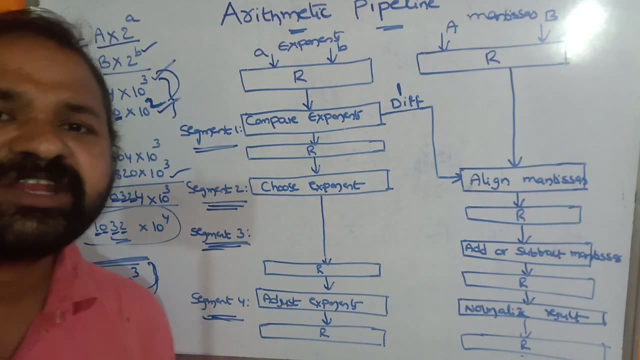 And let us assume that we performed the subtraction. After performing the subtraction, let us assume that we got this here as the result. So for subtraction also same thing. The first step is we have to compare the exponents. The second segment is alignment of mantises. 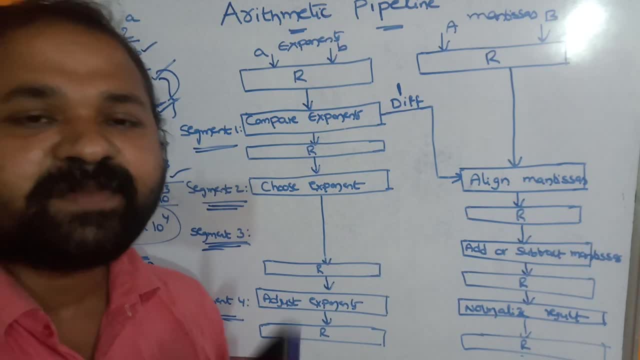 But the third one is subtract mantises. So when the mantises are subtracted then there is a possibility that we may get underflow. So whenever we get underflow then we have to perform shift left operation by decrementing exponent value. So what is underflow here?